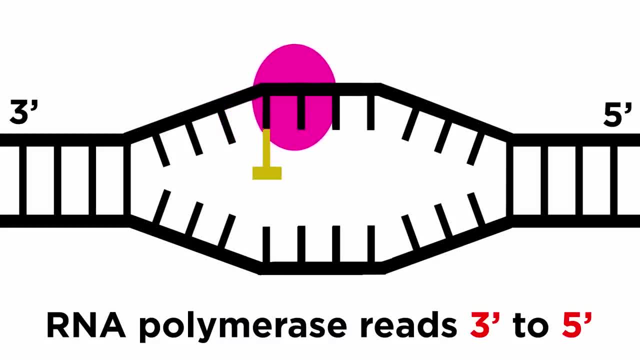 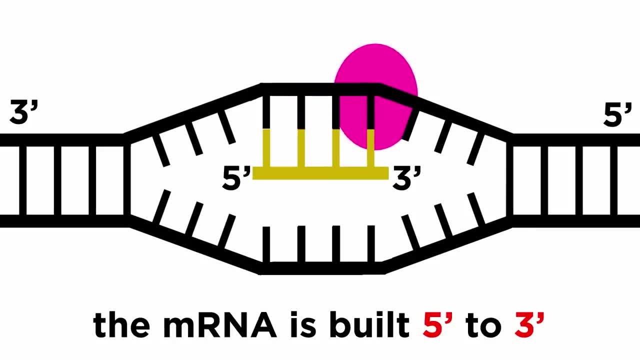 the mRNA as it goes, reading the antisense strand from three prime to five prime and generating the mRNA from the five prime end, attaching RNA nucleotides to the three prime end, as it goes. This is very similar to the way DNA polymerase synthesizes DNA as it moves along the template. 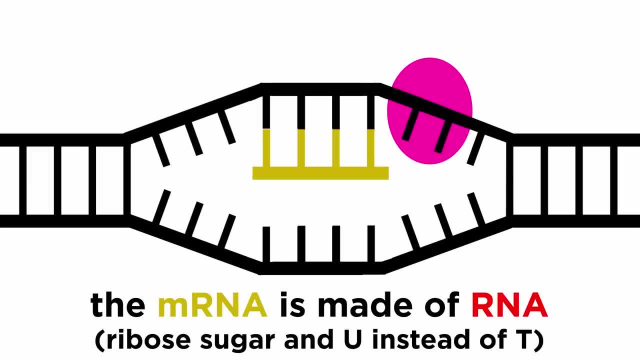 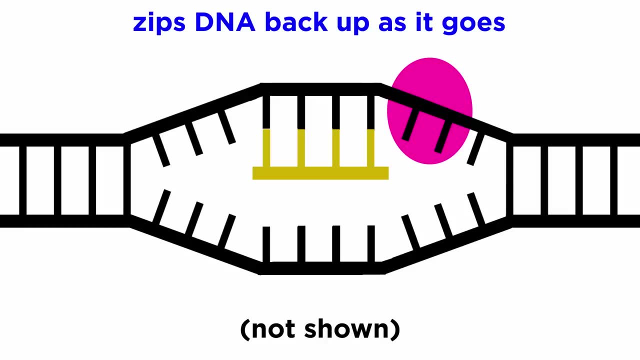 strand. The main difference here is that RNA is being synthesized Which, as we recall, will be ribose rather than deoxyribose, and it will have uracil instead of thymine. Unlike replication, RNA polymerase zips DNA back up as it goes, keeping only ten to twenty. 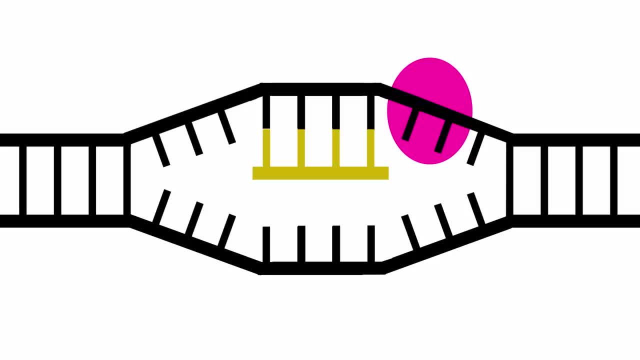 bases exposed at a time. Once RNA polymerase reaches the end of the gene, termination occurs. The enzyme detaches from the gene and the DNA is returned to its original state, But we have produced an mRNA. This carries with it the information in the DNA. 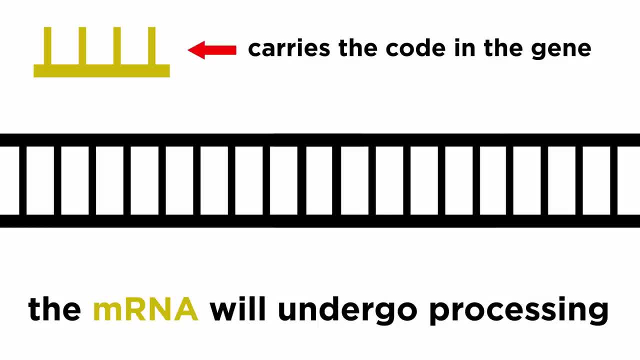 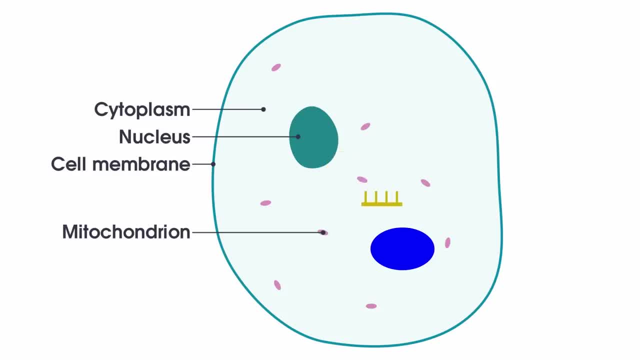 This is the DNA that is encoded in the gene And, after a few quick modifications during RNA processing, it will leave the nucleus, where all the genetic material, or chromatin is, and move into the cytoplasm where it will find a ribosome. 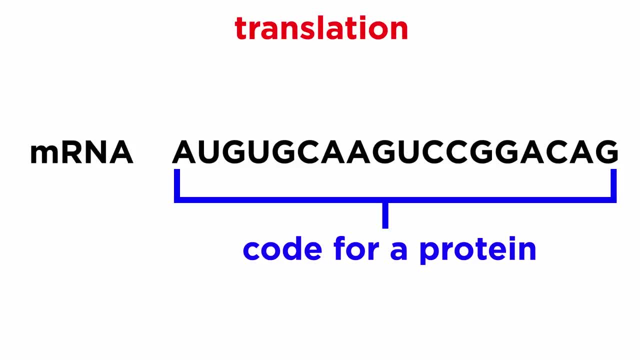 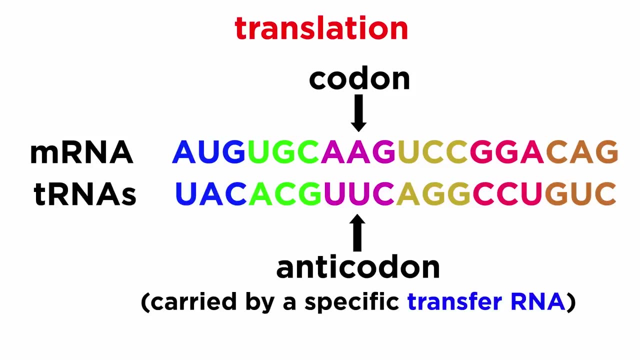 This is where translation occurs. During translation, the mRNA acts as a code for a specific protein. This happens because each set of three bases on the mRNA, which we call codons, will code for a specific anticodon Which will be carried by a specific transfer RNA or tRNA. 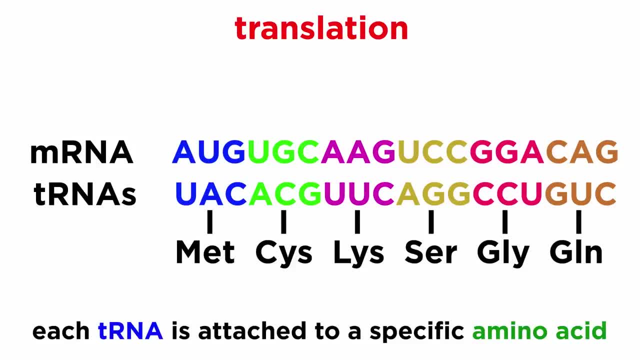 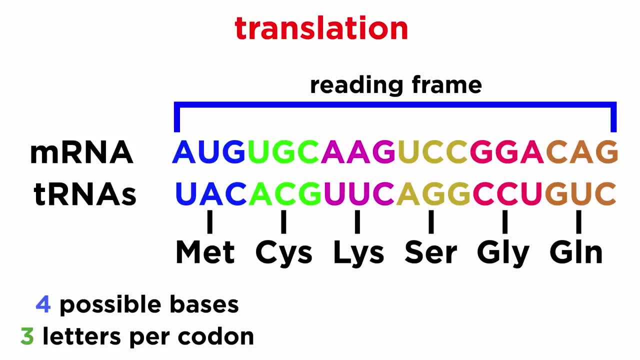 And each different tRNA is covalently linked to a particular amino acid. The arrangement of the nucleotides into these codons is called the reading frame. Since there are four bases and each codon has three letters, four cubed gives us sixty-four. 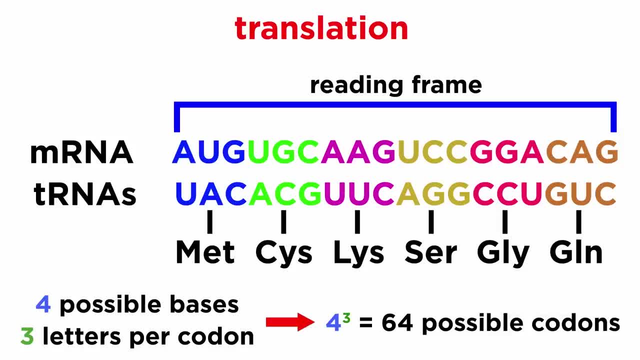 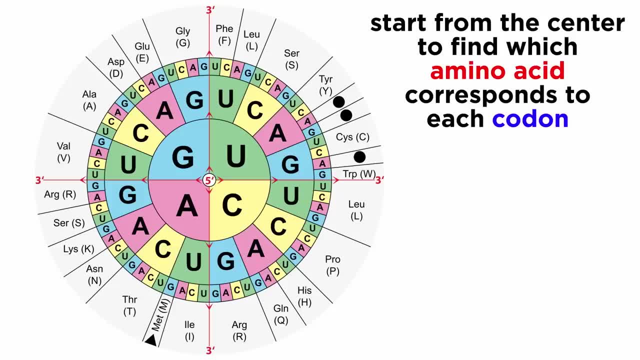 different possible codons, which is more than enough to code for all the amino acids we need. Here is a table of all the mRNA codons and the amino acids they code for. Notice that there is some redundancy with multiple codons resulting in the same amino. 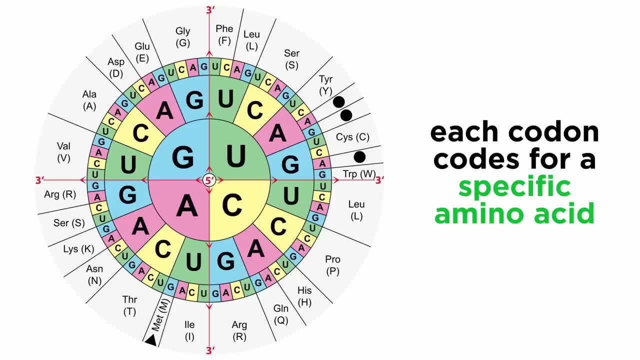 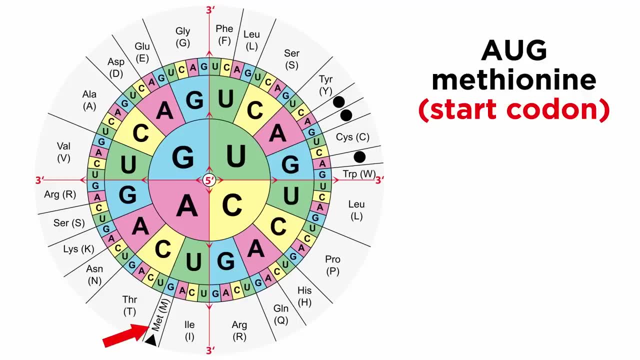 acid. But there is no ambiguity: Each codon corresponds to a particular amino acid. Notice also that some of these codons are special: AUG is the start codon, which initiates translation by coding for methionine, And these three are stop codons. 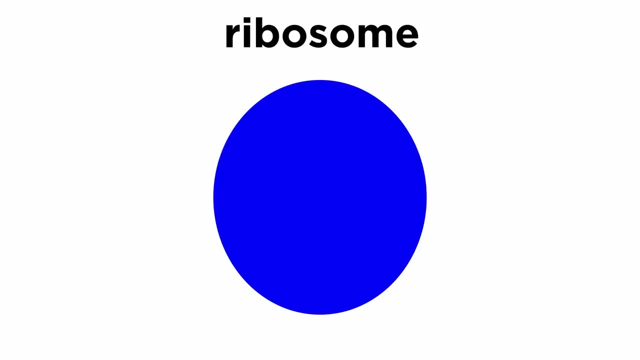 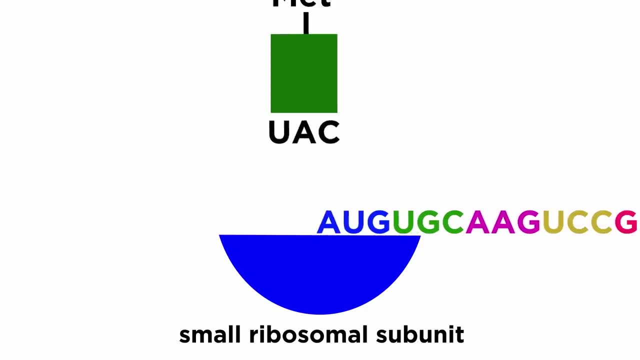 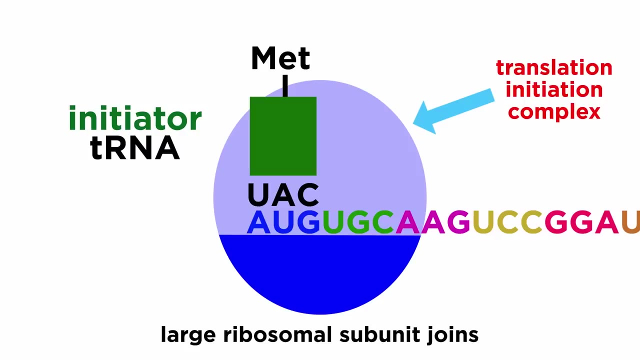 These are the ones that terminate translation. Translation will occur inside a ribosome. The small ribosomal subunit binds to an mRNA and an initiator tRNA, which adheres to the start codon. Then the large ribosomal subunit joins to complete the translation initiation complex. 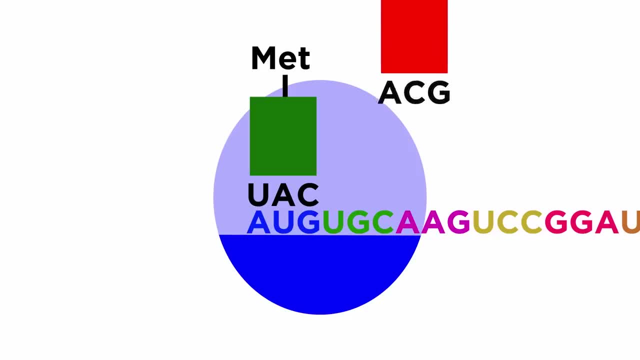 Then the tRNA that corresponds to the next codon. after the start, codon will enter the ribosome. This will carry with it an amino acid which becomes covalently bound to the methionine from the initiator tRNA. The first tRNA detaches and leaves the ribosome. Which is just the base. the officer will then take it and outline this, Which leaves the ribosome. after the start: codon. And then you have these three. If we make a r that complete the compression between these two isotopes, Then the first tRNA isrowed in the next codon. after the start: codon. 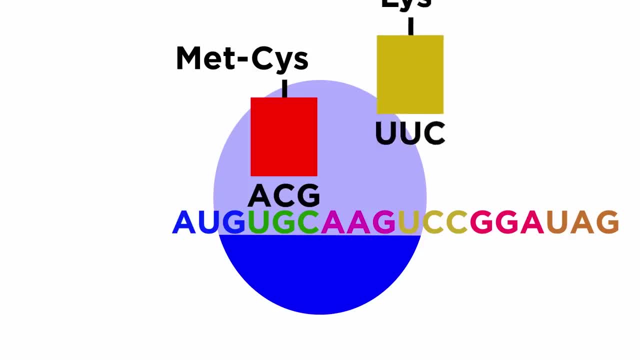 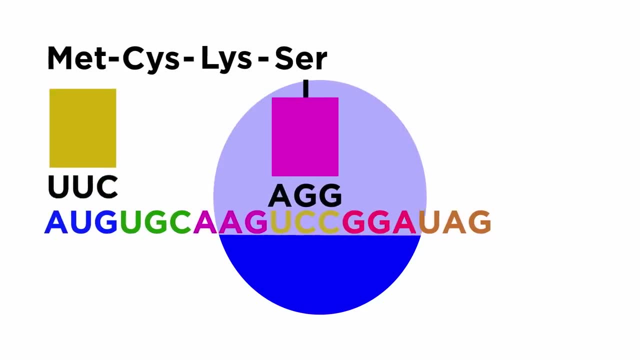 which has shifted over, making room for the next tRNA. The new amino acid links to the first two and this process continues all the way down the mRNA, As tRNAs enter and exit the ribosome in a sequence that is dictated by the codons. on. 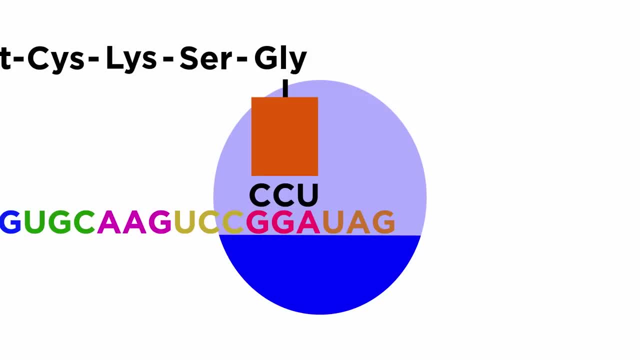 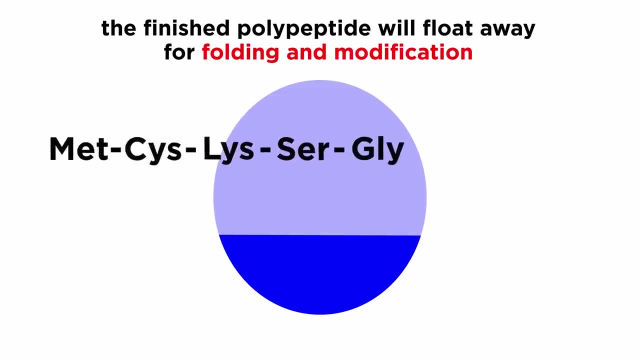 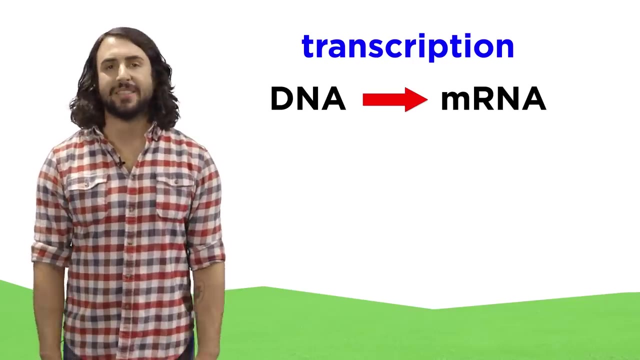 the mRNA, a polypeptide chain will grow. This continues until a stop codon is reached, at which point the completed polypeptide will swim away, most likely entering one of the cell organelles for folding and further modification. So, in this two-step process, DNA is transcribed into an mRNA and then this mRNA is translated. 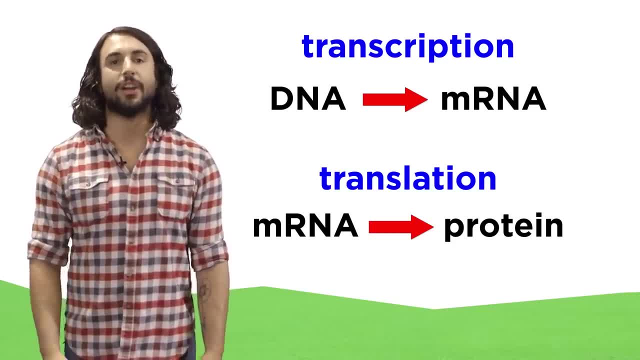 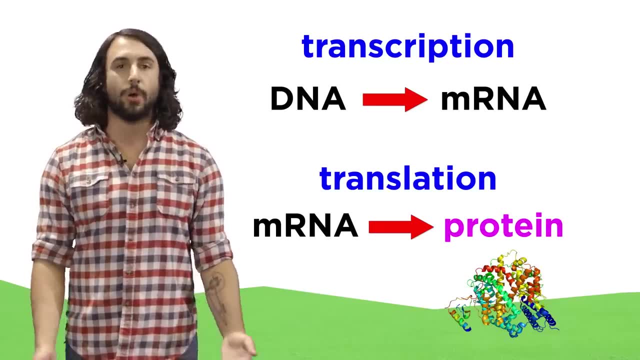 into a protein, all simply by obeying the base pairing that occurs in nucleic acids And since every gene codes for a specific protein, and proteins make up most of what you are, from your muscle tissue and organ tissue to all of your receptors and enzymes. 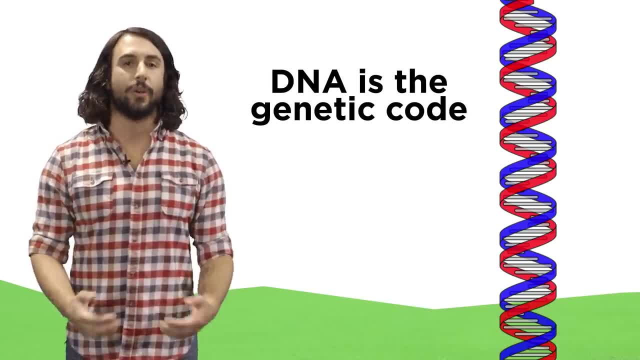 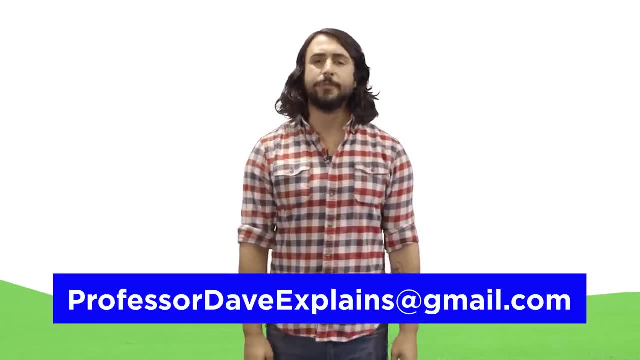 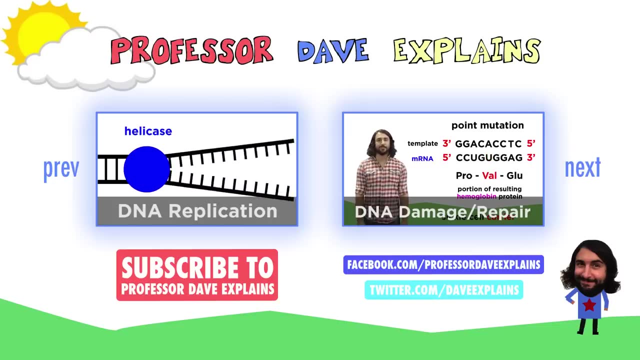 this is how DNA carries the code for a living organism. Thanks for watching, guys. Subscribe to my channel for more tutorials and, as always, feel free to email me professordaveexplains at gmail dot com. I'll see you next time. Bye.